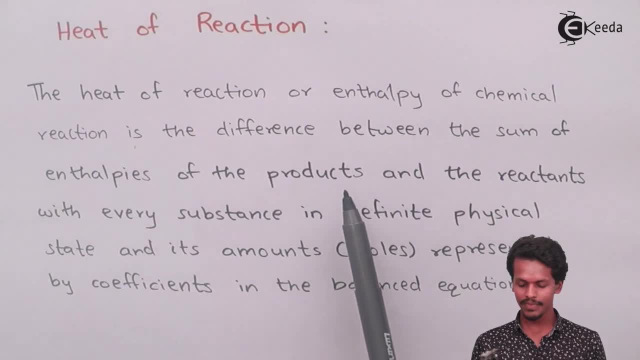 the sum up of all the enthalpies of product and the sum up of all the enthalpies of the reactant, with every substance in a definite physical state and its amount, that is, the number of moles represented by coefficients in a balanced equation. So the enthalpy of a particular 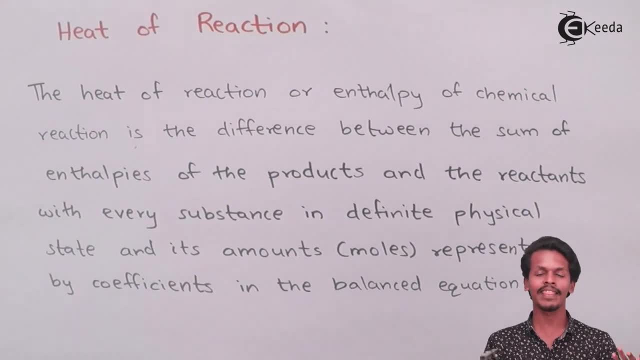 reaction. it is very much simple to understand. it is nothing but the enthalpy of the product, the sum of enthalpy of the product and the minus the sum of enthalpy of the reactant. and if we do this thing, then what are? whatever, the amount that we get will be the amount of the energy or the enthalpy that 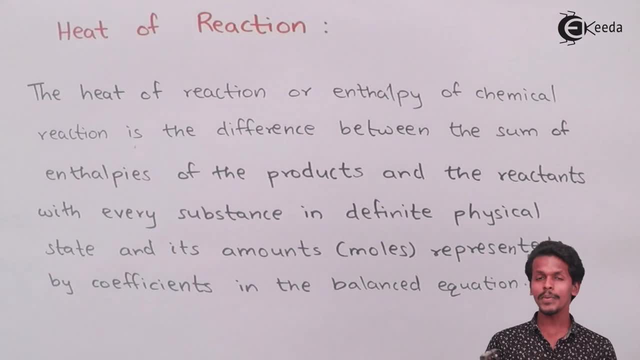 has been changed during this process. So let me talk more deep about this thing is that we should always consider that the reaction that we have or on which we are studying, that should be thermodynamically or that should be stoichiometrically balanced. So if that has been a balanced and then it would be very much. 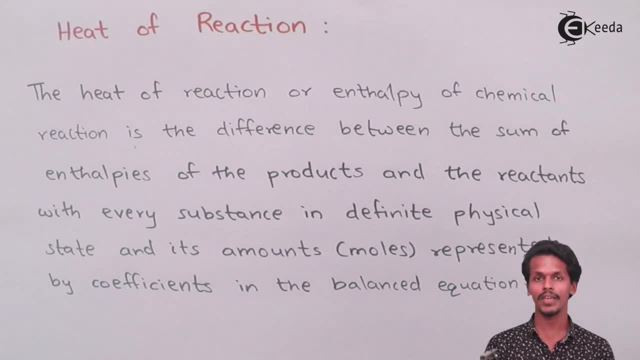 easy to understand because this deals with the change in enthalpy when all the reactants or all the products have a particular coefficient, that is, the stoichiometry associated with it, and during that, whatever change we observe, that would be a precise change in enthalpy during that. 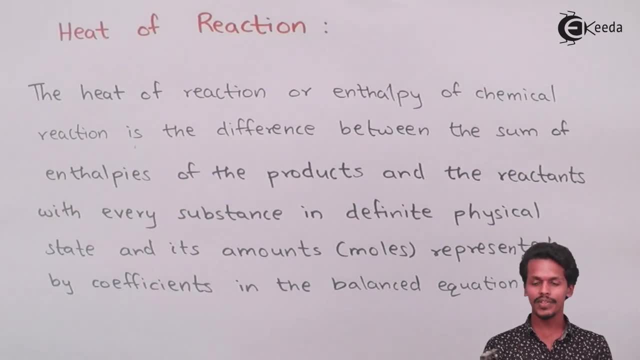 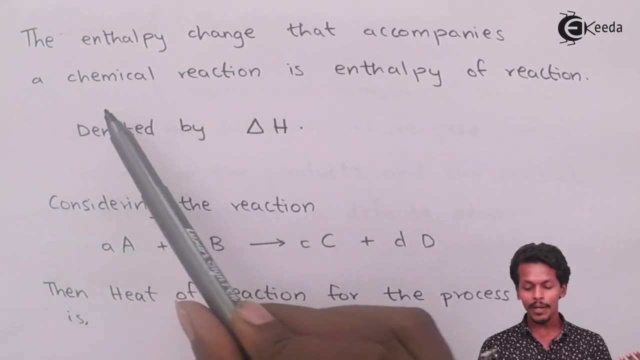 process. So let me give you more detail about this thing that what is actually heat of reaction. it is a very simple concept, but is the enthalpy change that accompanies a chemical reaction? is enthalpy of reaction means in a chemical reaction, the change that it occurs? 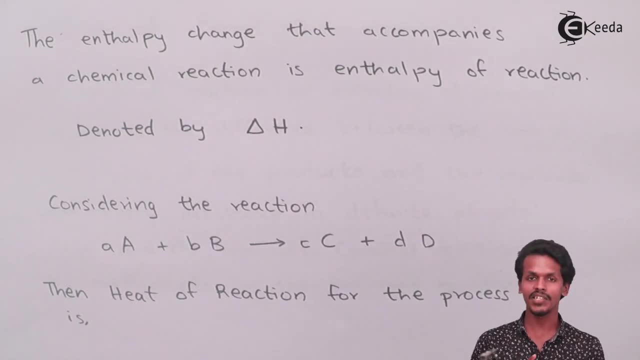 that the enthalpy change that occurs for a chemical reaction, that is nothing but the enthalpy of the reaction or heat of the reaction. It is denoted by delta h and that delta h can be positive, can be negative. we are going to talk about it later, but we should. 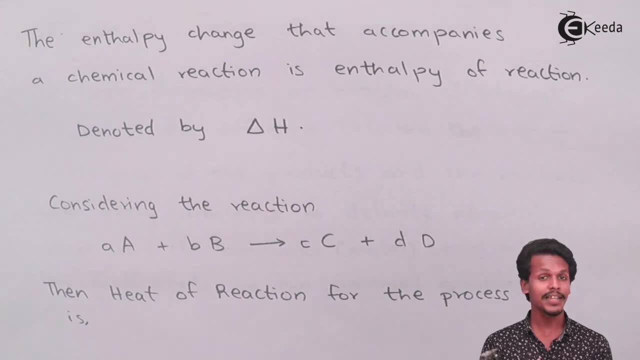 also talk about how can we calculate the delta h of a particular reaction. So suppose we have a reaction like a modes of a plus b modes of b. that gives us c modes of c and d modes of d. So this is the reaction that we have and in this case, what we 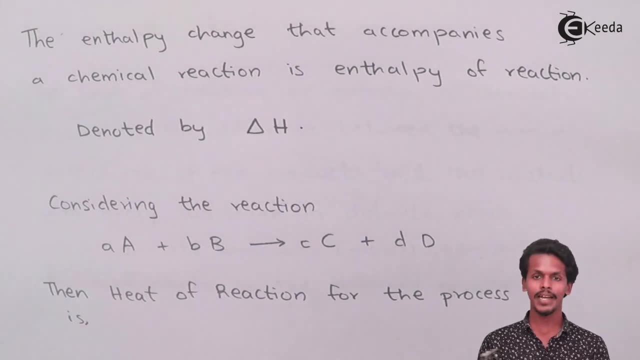 observe is that the a and b, the both are in reactants, while the c and d are the products, and the small a, small b are the coefficients or the stoichiometric coefficients of the reactants a and b respectively, while that of the small c and small d are the stoichiometric coefficients of 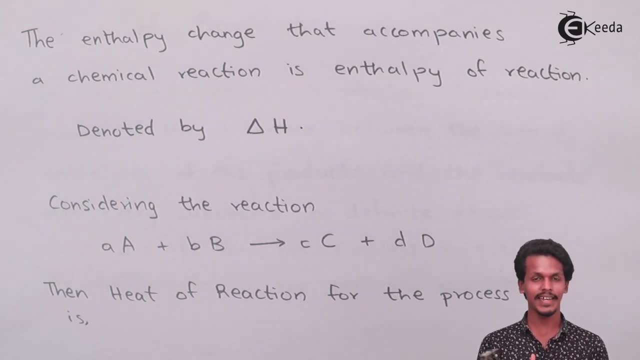 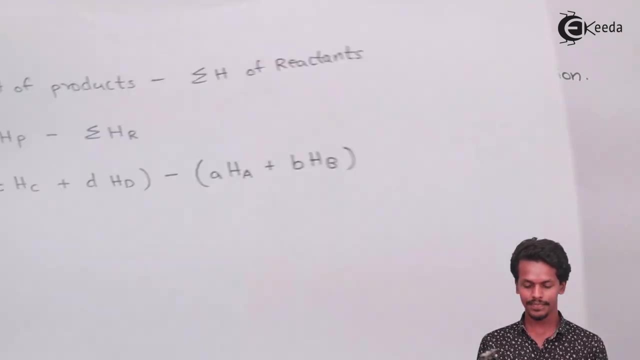 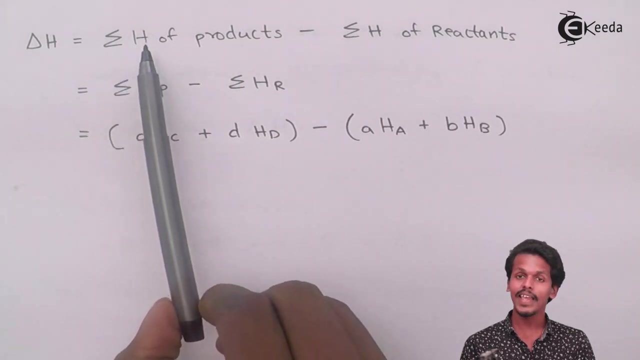 that the number of modes of product, that is, c and d respectively. So therefore the heat of reaction in this process can be easily calculated, as by this formula. The formula is: that is, the delta h is equals to summation of enthalpy of the product minus. 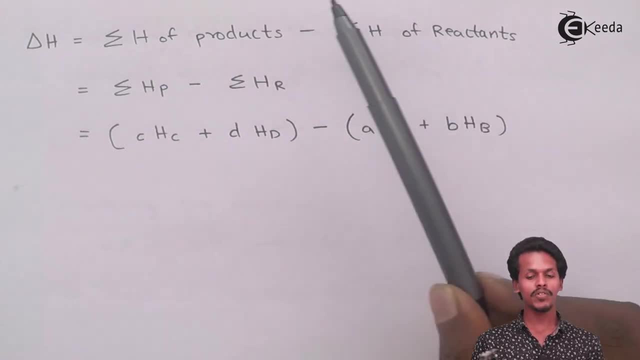 summation of enthalpy of the reactant. So this can be also be written as a summation of hp, that is the enthalpy of the product, minus summation of hr, that is the enthalpy of the reactant. So, since the product input, 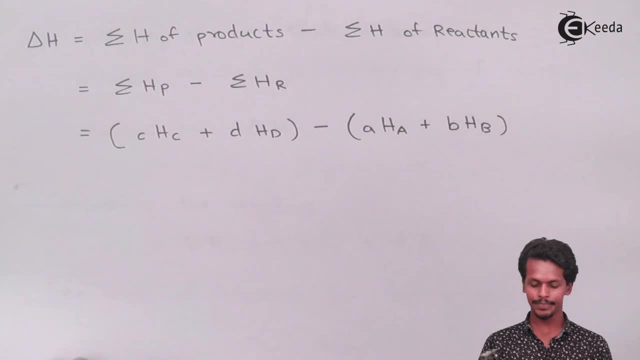 what was been. we have observed. we have observed that it has c modes of c, while b modes of t. So similarly, here also, we could see that. now, how to calculate this thing? So, because small c was the stoichiometric value. so that's the reason we are now multiplying. 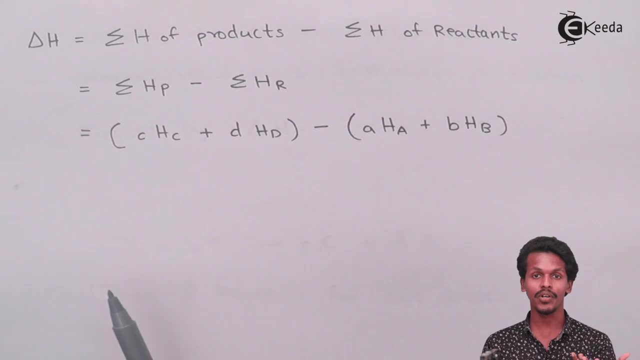 Class a 2 was the最後. in it we had the stoichiometric value with the enthalpy of the product c. so therefore c will be multiplied by the enthalpy of the product c plus d was the number of modes of the capital d that we had. suppose it is product. So again, it will be multiplied by. 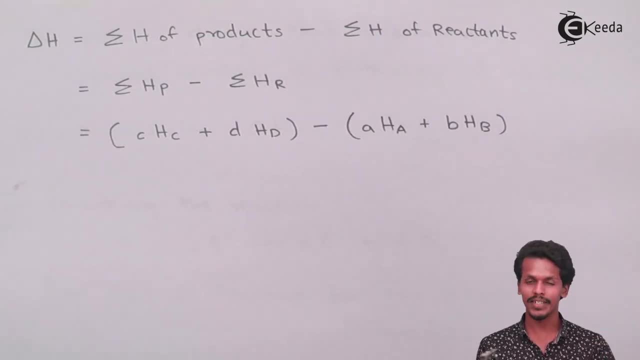 the enthalpy of d. so this is basically the sum of of the product that we had minus a. modes of A now will be multiplied by the enthalpy enthalpy of A plus B. moles of B now will be multiplied by the enthalpy of B. so 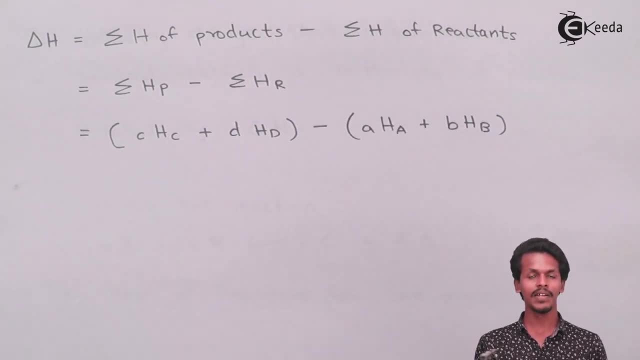 this will be the sum of the reactants. so if we do this subtraction or if we make out a difference between them, so that will be nothing but the enthalpy of the reaction. for example- I have an example in my mind, suppose if it is two times of: 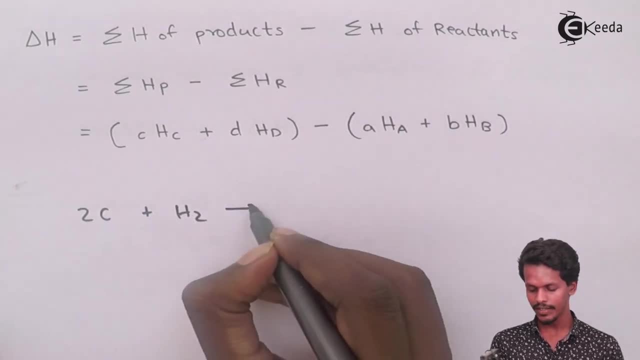 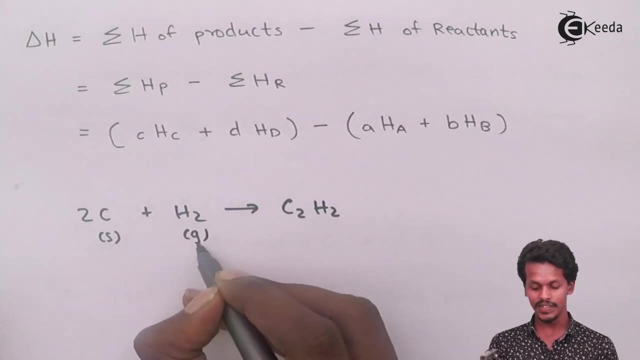 carbon plus H2, so it will give me C2H2, and again carbon is present in solid, while hydrogen has been present in a gaseous state and again- this is ethene that we will get- again it will be present in a gaseous state. so in this, 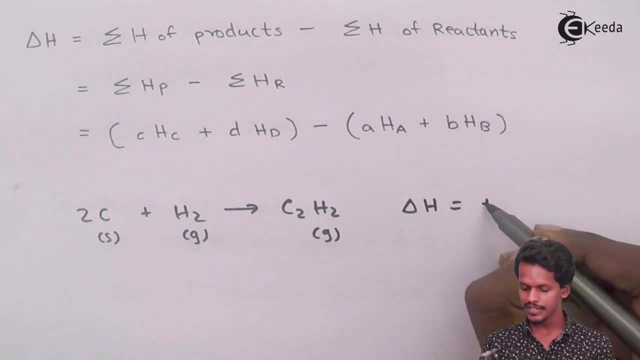 case the delta H which was found to be, it was around somewhere plus two to six point zero kilojoules per mole. so this implies what? so this is nothing but the the. so this implies what? so this is nothing but the heat of reaction, which means that, suppose if carbon and hydrogen, the both 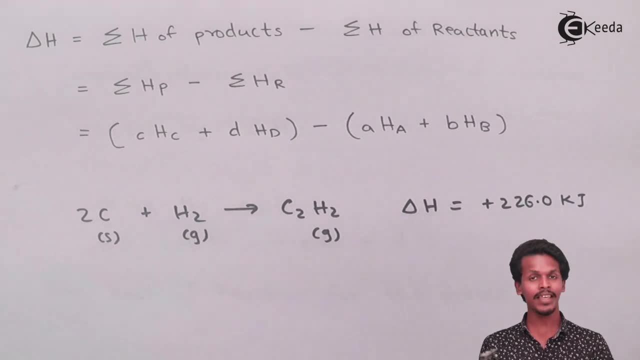 comes together to each other and they react with each other so as to form ethene. but anything in this thing we should also mention and we should also observe that the stoichiometric values are also being given. that is, two moles of carbon now will be engaged with the H2 molecule so as to form one mole of. 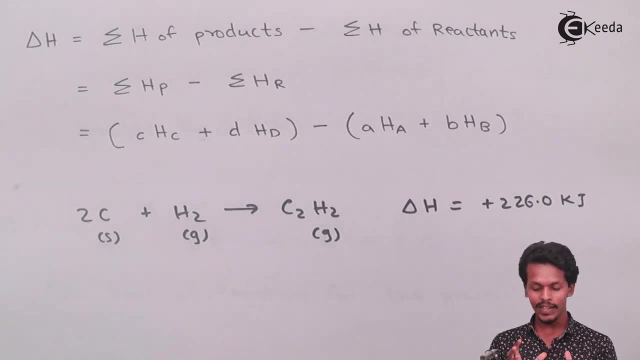 C2H2, that is ethene. so in this, for to keep in this mind, then, only the value of delta H has been enough for this reaction. it was plus two to six point zero kilojoules means this much amount of energy has been released when carbon was being reacted with hydrogen so as to 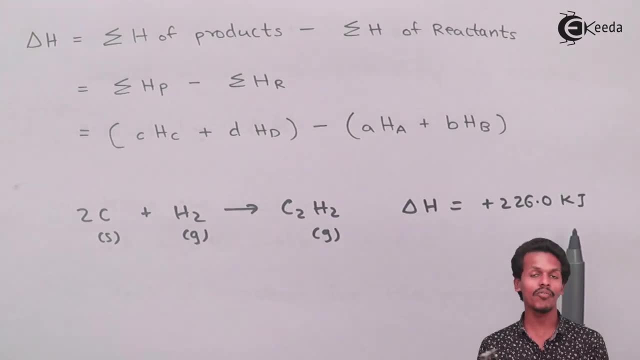 form ethene. so this is nothing but the heat of reaction or the enthalpy of the reaction. but this is for the particular reaction, that is, for formation of ethene. but for different reaction it would have a different value and it will depend that whether the value will have a positive magnitude or a negative. 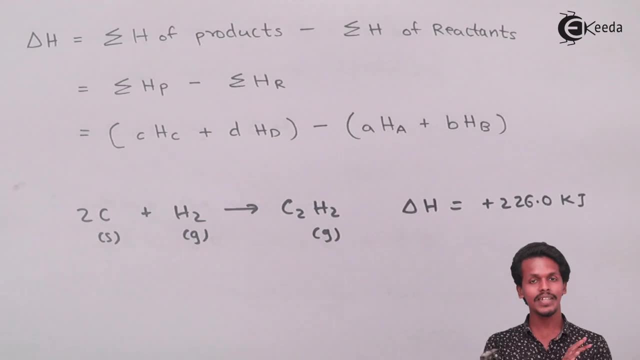 magnitude. so talking about the next one also. so this was related to the state, it was related to the enthalpy of the reaction. but yes, we have also another condition in which the same enthalpy of the reaction can be calculated, but the condition will be different. and what is the condition? let us talk about that. so 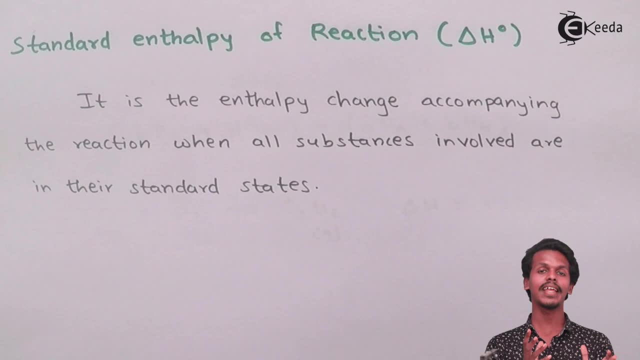 now we are going to talk about standard enthalpy of reaction. so the difference between the enthalpy of a reaction and standard enthalpy of the reaction is that in standard enthalpy the condition are set to be or are set to be in a standard values, for example the pressure which is 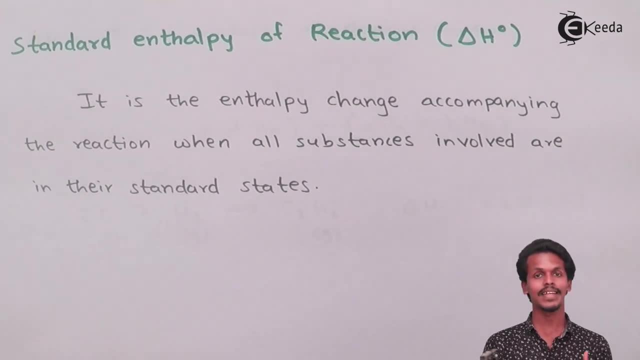 basically, it should be set at 1 atmosphere. the temperature: it should be set at 25 atmosphere. so that is nothing but the standard enthalpy of the reaction that we have suppose in this thing, so as to learn the definition of this thing. it is nothing but the enthalpy change accompanying the reaction.